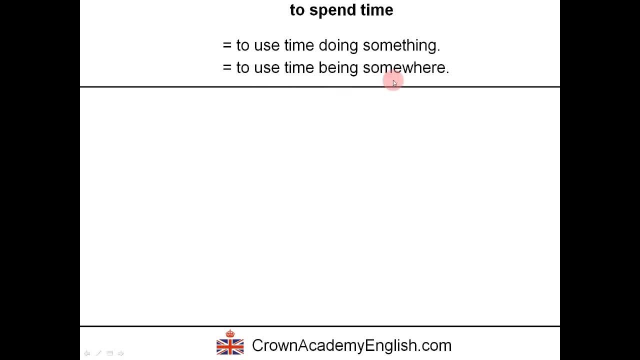 Also it means to use time being somewhere. Okay so when we go somewhere. So two examples: Jane spent six months studying for the exam. So this is the past tense, the past simple form of spend, Spent with the letter t. So in the past, Jane spent 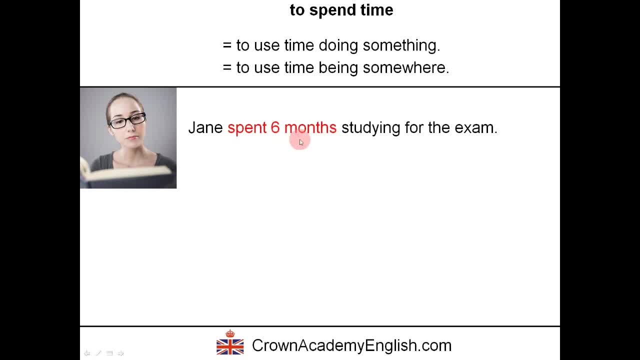 followed by the duration of time, the period of time. Jane spent six months studying for the exam. And notice, here we have a present participle, the ing form of the action of the verb. Okay, so we could also say: Jane spent two weeks studying for the exam, Jane. 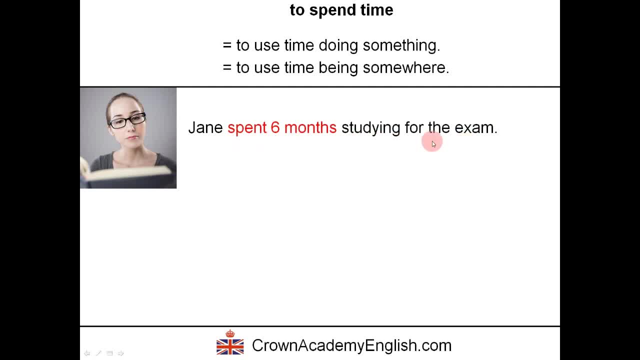 spent three days studying for the exam. Okay, we could simply say Jane spent some time studying for the exam, But we usually say spend followed by a period of time. When I was a student, I spent nine months living in Paris- Okay, so I spent- followed by the duration of time. 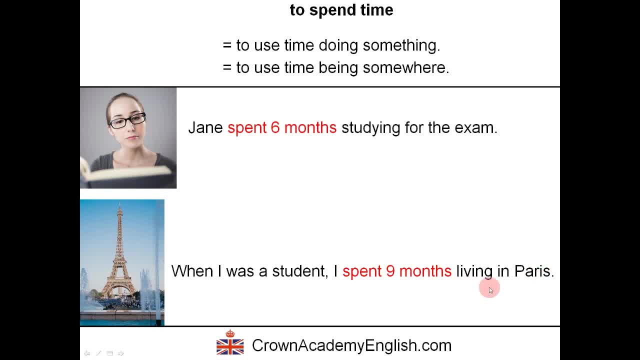 Nine months living in Paris. And again here we see the ing form of the verb of the action. This is a true story. by the way, I really did spend nine months living in Paris when I was a student, So I speak French. 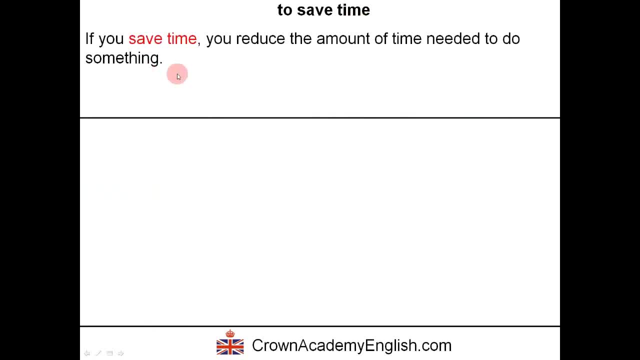 To save time. So if you save time, you reduce the amount of time needed to do something. So when you save time, you are able to do something in less time. Jane asks: do you walk to school? And Mark replies: no, I take the bus to save time. 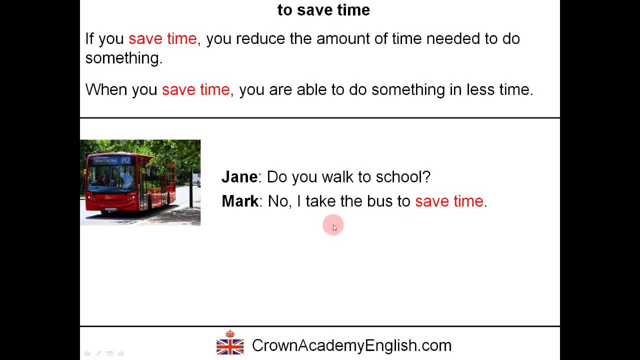 To save time? Okay, because it is quicker to go to school by bus, then that means you save time because it's quicker than walking. Okay, it takes less time. Claire saves time by eating lunch at her desk. By eating lunch at a desk, So Claire saves time. 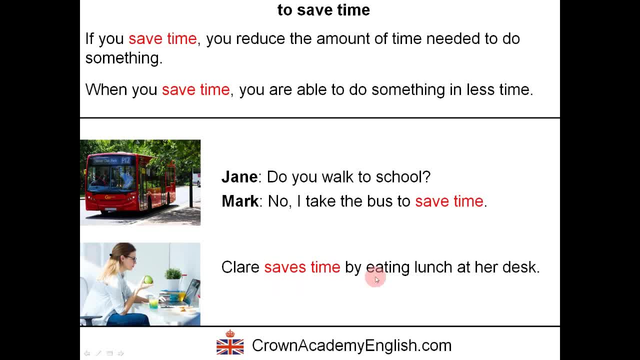 And why does? how do we save time by doing this? Well, it's because Claire is doing two things at the same time: She's eating lunch and she is working, Okay, so by doing two things at the same time, you save time. 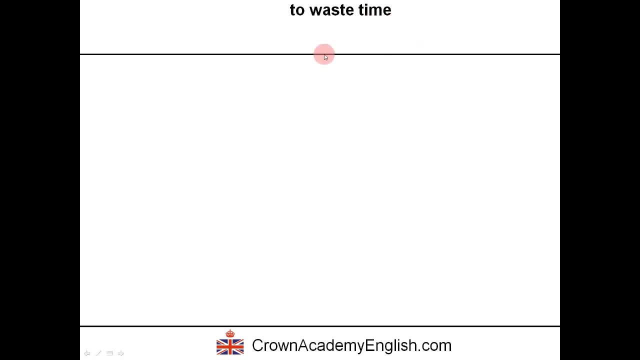 To waste time. Okay, so this is: if you waste time, then it's it's not a good thing And it means to not make good use of the time that you have. So if you waste time, then you are not being efficient. Okay, you are not making a good use of the time. 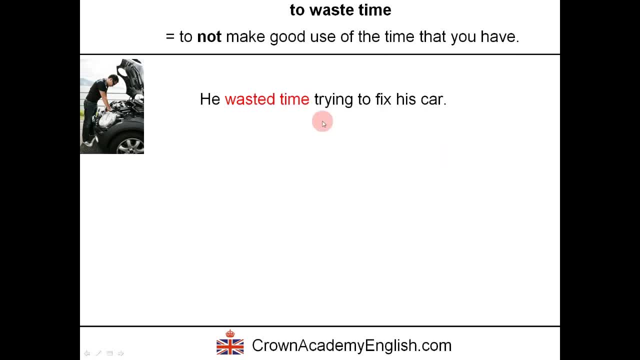 Here is an example: He wasted time trying to fix his car, So he doesn't know anything about cars. He doesn't know how to fix a car, So he's wasting time by trying to fix it. Okay, because he should just call a mechanic. He should ask someone else for help. 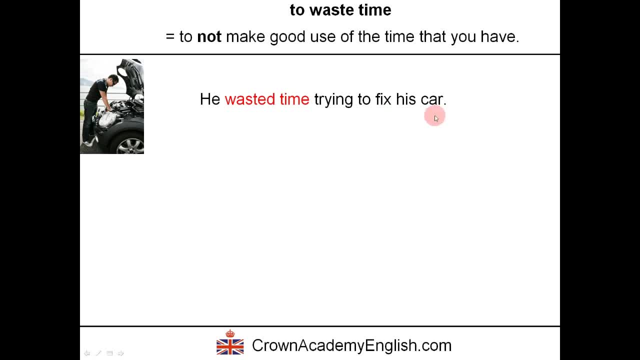 Because he doesn't know what he's doing, So he's wasting his time. Okay, He's not making good use of his time, Because he'll never fix it. Mark wastes four hours a day playing video games. So Mark wastes four hours a day playing video games. 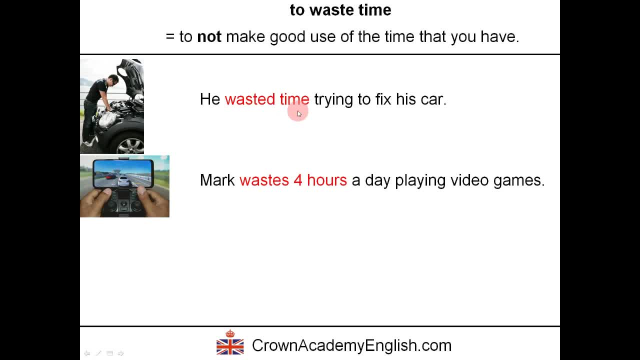 So notice, with this expression we can either say wastes time, or we can say wastes, and we can specify the duration of time. So wastes four hours, wastes two days, wastes a week, Okay. so put this example: Mark wastes four hours a day playing video games. 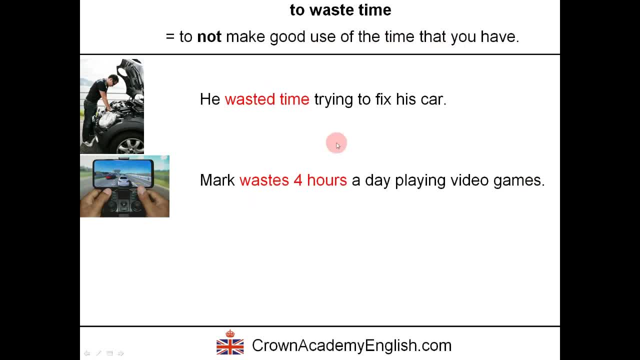 because it is not a good use of his time. I think perhaps Mark should be doing something else. He should be maybe sleeping or working. And there is also a noun. This is the verb to waste time, but we also have a noun: a noun. 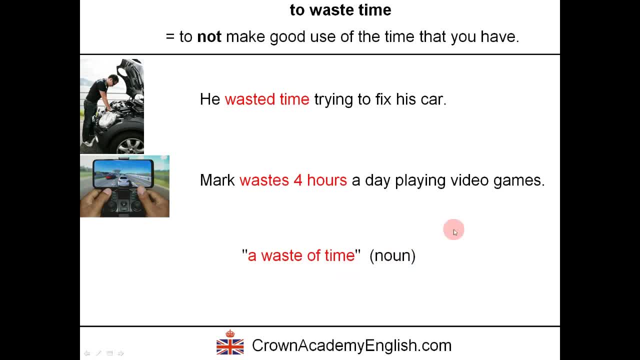 phrase Something is a waste of time, And here is a very common example: a meeting, So this is a meeting at work. Nothing was decided during the meeting. It was a waste of time. So the meeting was a waste of time. This is. 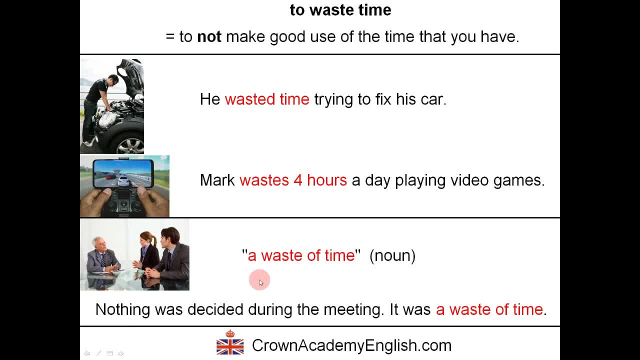 very common in offices. You often have a meeting that goes on for hours and hours and hours and nothing is decided, and at the end of the meeting you think, wow, this is a waste of time or this was a waste of time. You can also say this was a. 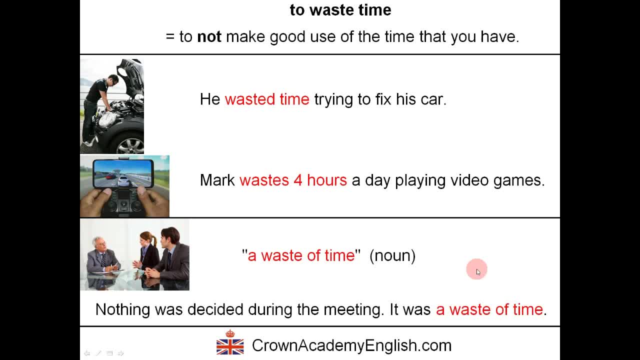 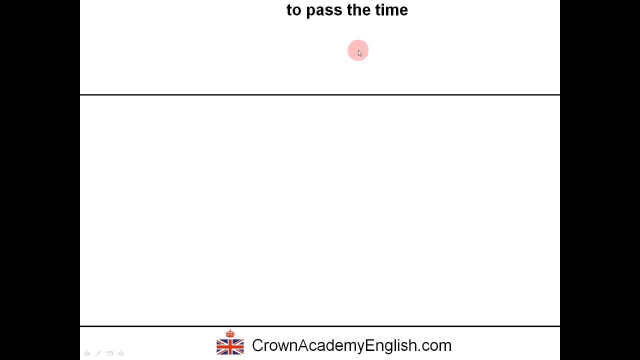 waste of my time. Okay, to pass the time. so this is different to SPEND time. This is a, a, a difference expression, And it means to use time to occupy yourself, to keep yourself busy, to do something with the time, And it also means to use time you. 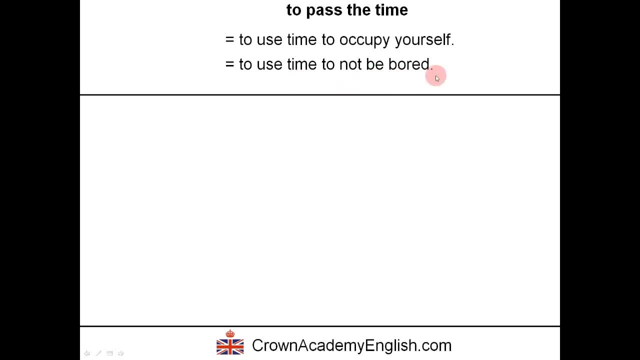 time trying not to be bored. To not be bored, So to occupy yourself. Example: the context is: Mark and Jane are waiting for a flight at the airport And Jane suggests let's play cards to pass the time. And Mark says: good idea, So they're. 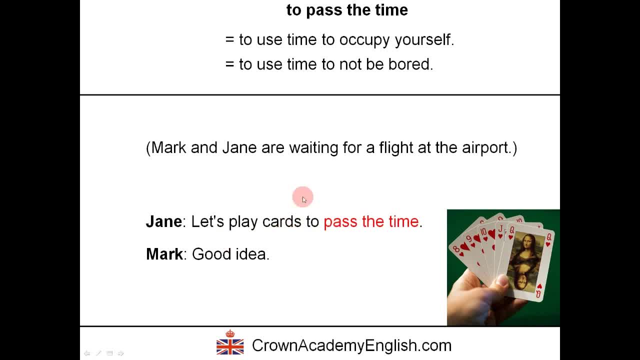 bored. basically, They have three hours, four hours to wait for the flight and they have nothing to do. They don't know what to do. They have to sit there, and so they are looking for an activity to pass the time And they decide to play cards. 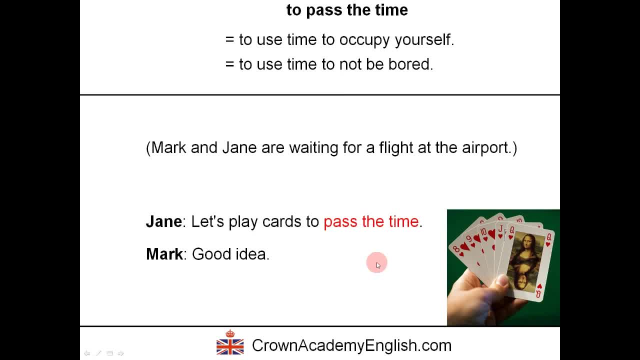 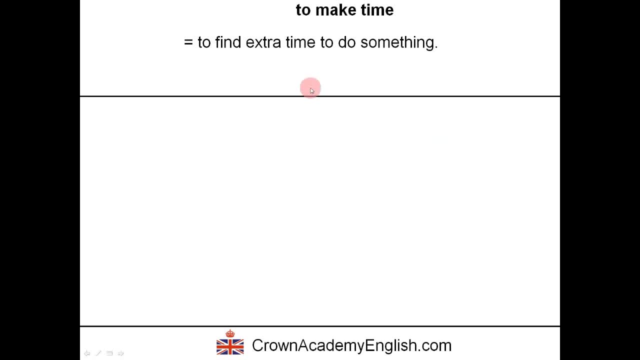 to pass the time, To make time. So this means to find extra time to do something. Okay, so when we are making time, we are talking about things like priorities. Making something a priority, So yes, so to make time, it's. 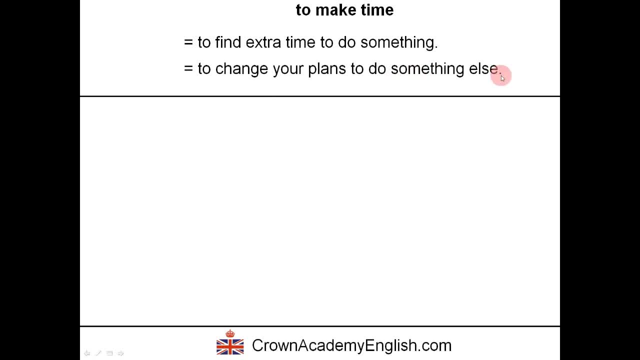 when we change your plans to do something else. So the manager says: I want you to finish the reports, But Mark says: I don't have time to work, work on the reports". Well, the manager says: well, you must make time, You must. 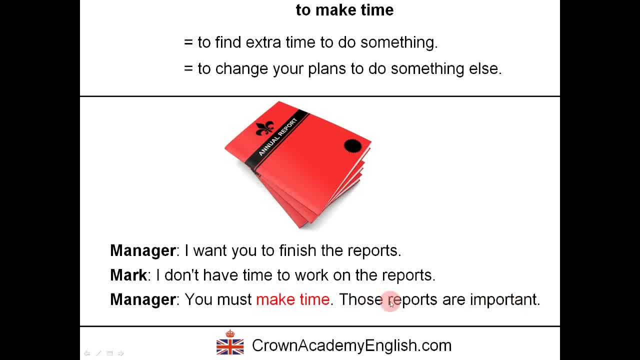 make time. Those reports are important. So the reports, they are a priority. and the manager is saying: you must make time for the reports. So stop, stop doing what you're doing already and start working on the reports. So make time for the reports, Make the reports a priority. 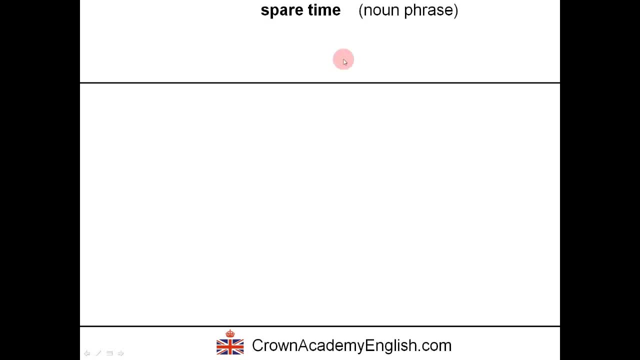 Spare time. This is a noun phrase. Another way of saying this is free time. So free time or spare time, And it means time when you're not working. So time when you're not working or time when you are not studying, maybe. 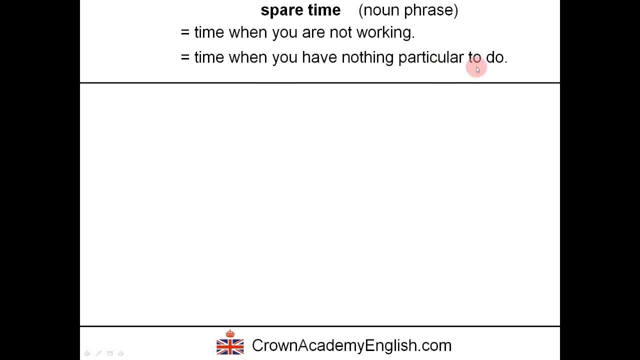 It's time when you have nothing particular to do So with this expression, with this noun phrase, we have a very common question when you are getting to know someone. This is a very common question in English: when you're talking to someone, What do you like to do in your school? 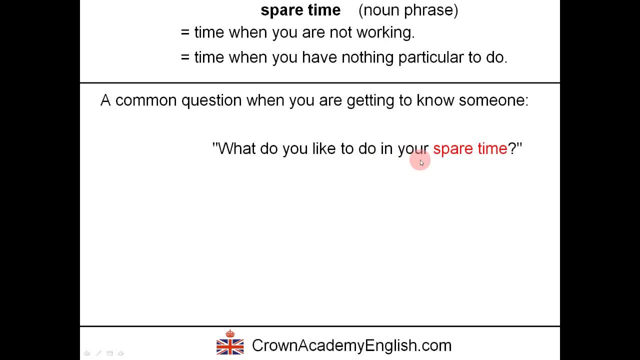 In your spare time. What do you like to do in your spare time? So this is a different way of asking: what are your hobbies? Okay, Because we do our hobbies in our spare time. So if someone asks you, what do you like to do in your spare time, 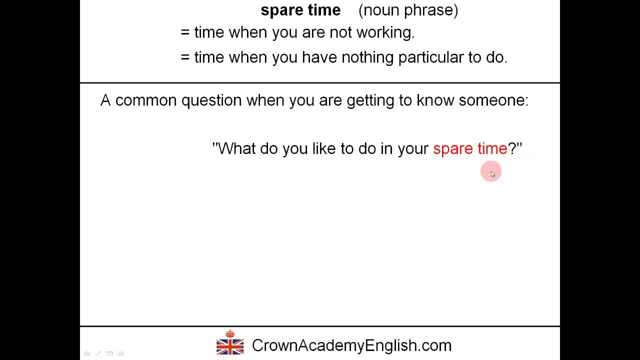 they are asking you what, they're asking you for your hobbies. So a common, you know an example answer would be: I enjoy playing the guitar. Or maybe you would say: I like watching football. I like playing football, I like going to the cinema. 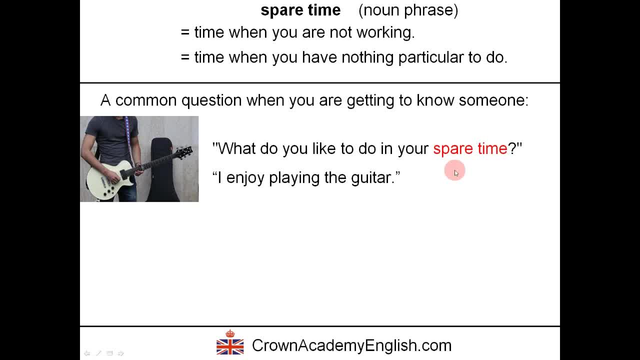 Okay, Because you do all of those things in your spare time When you're not working. Claire asks: What did you do this weekend? David replies: I had some spare time, so I did some cooking. I had some spare time, So this is the past tense. 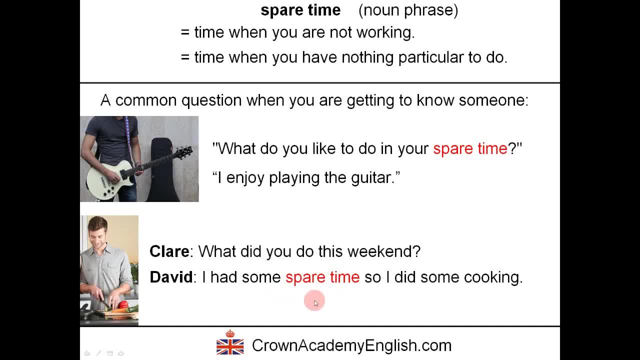 So in the present tense you can say I have some spare time. This is the past. So David says I had some spare time. Notice, we have some spare time, But time here is singular, In the singular form. Why is that? 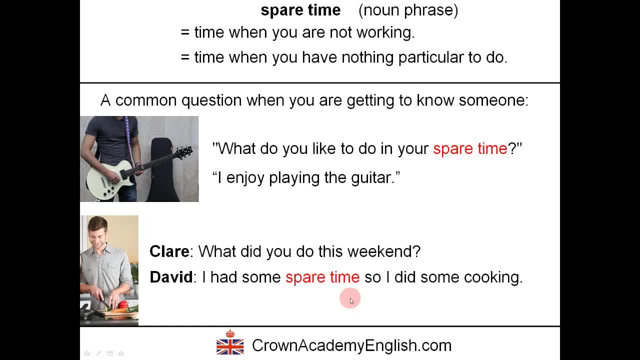 Well, this is because the word time is an uncountable noun, Uncountable noun, Okay, And if you don't know what that means, then there is a link at the end of this video to my video explaining countable and uncountable. 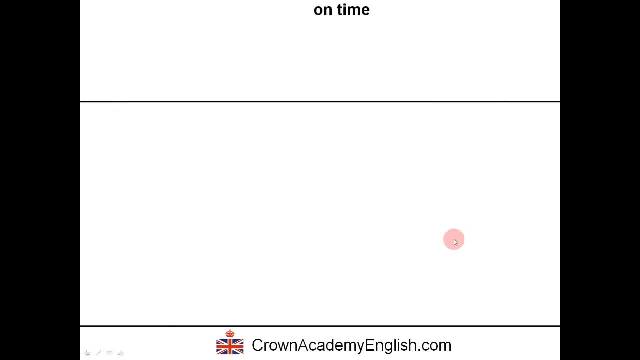 nouns On time. We use on time to describe timetabled events or scheduled events, Events that happen at a fixed time, And it means well on time means that something happens at the scheduled time. It is punctual, It occurs. 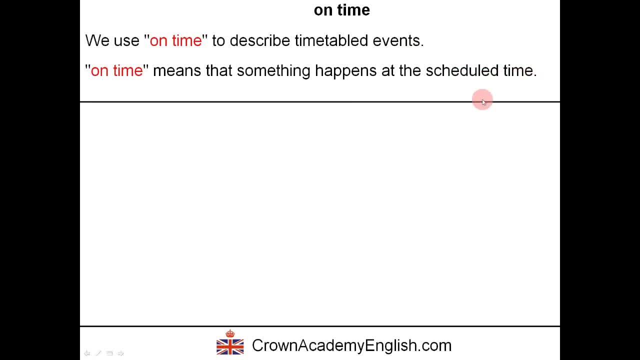 at the correct planned time, The time that we expected. And a very, very common example is a train. The train arrived at the station on time, On time. So if the timetable, if on the timetable, the train is expected to arrive at nine o'clock. 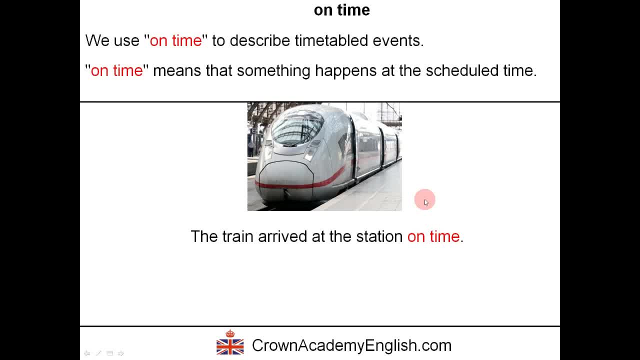 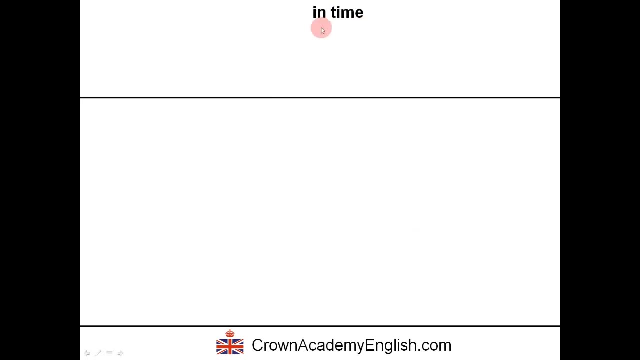 and if the train arrives at nine o'clock, then we say the train was on time. Okay, Now we have a different expression in time, And this is slightly different. In time means that we are not late, It means that we have enough time. 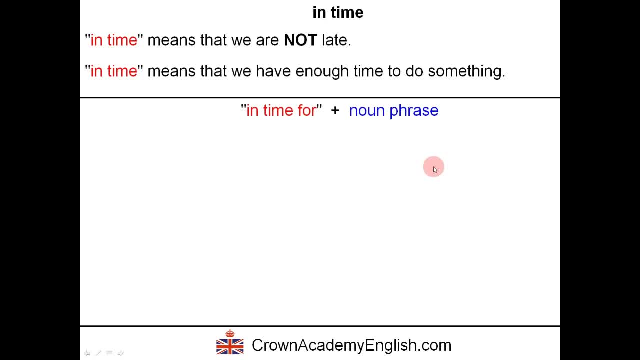 to do something And we have two forms. There are two, yes, there are two expressions with two different forms. We have in time for, followed by a noun phrase, And an example is: we arrived in time for the concert. We arrived in time. 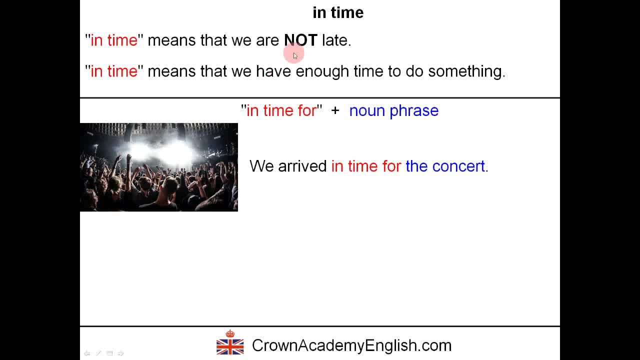 for the concert. So this means that we were not late for the concert. We arrived before the concert, In time for the beginning. Okay, So we had enough time to watch and listen to the concert, And we can also say: in time followed by. 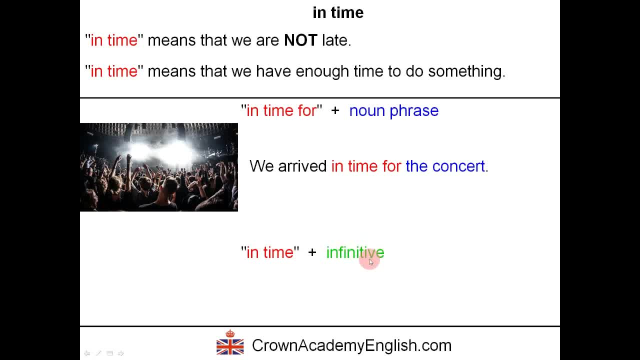 the infinitive of a verb. So the infinitive of a verb is to followed by the base form. Example: She arrived in London in time to visit the art gallery. In time to visit the art gallery. So this is the infinitive. 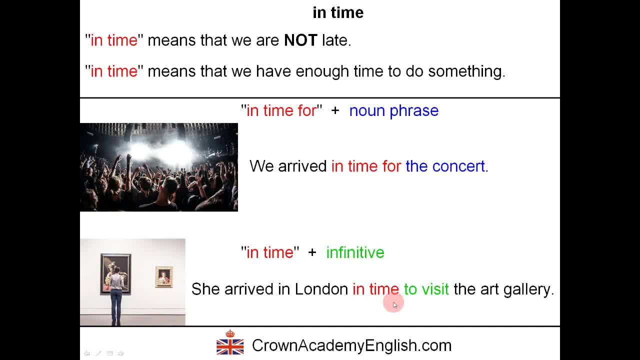 To visit. This means she arrived in London before the art gallery closed. Okay, If she was in time to visit the art gallery, then this means she arrived before the art gallery closed. So in time to visit, We could say she arrived in. 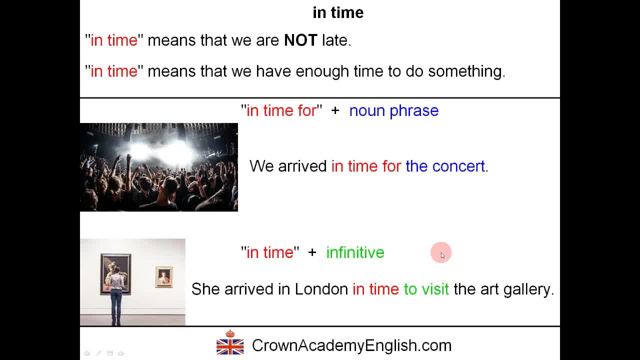 London in time. in time to visit a park, or in time to find a hotel, Okay, So lots of possibilities with this expression. So in time for, followed by a noun phrase, or in time followed by the infinitive. Okay, There we are. That's the.